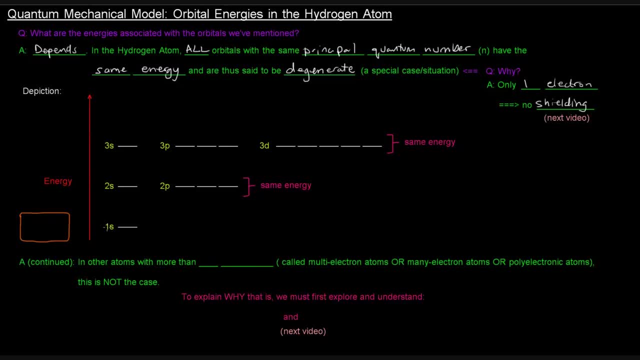 It's a very special case. So there's only one s, there's only one orbital in the first shell. In the second shell there's a 2s orbital and the 2p orbital In the hydrogen atom. they have the same energy. 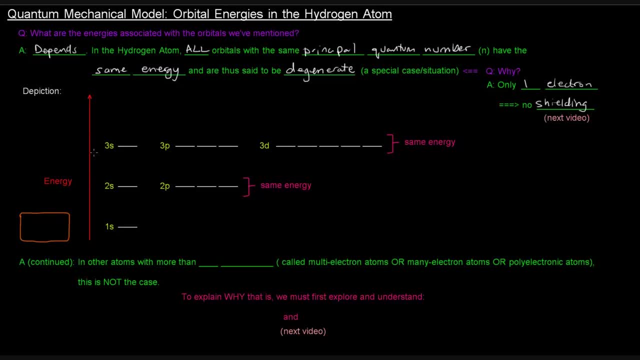 They have the same level of energy. If you go up to the third one, we got a 3s, The 3s, the 3ps and the 5, 3d orbitals and they're all at the same energy level. okay, 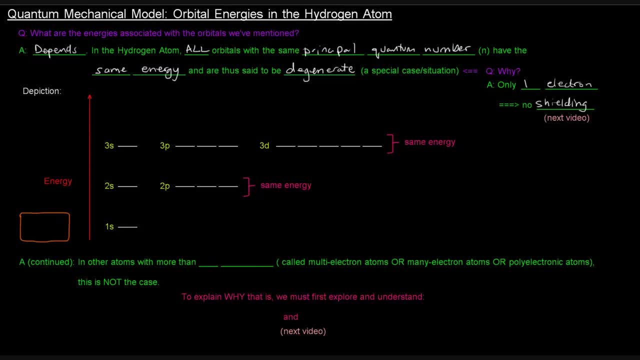 So if you have a hydrogen atom has one electron. if it's in its ground state, which means it's not excited, then it has one electron in the 1s orbital And it's considered at the ground state. It kind of looks like that okay, where all these other orbitals are at the same energy level. 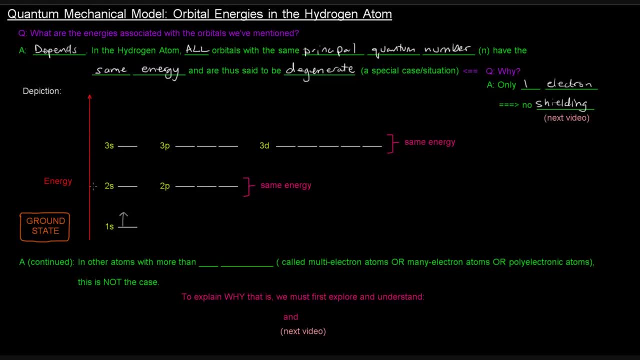 If they're the same, they have the same energy. If they're at the same energy level, they have the same principal quantum number. So if I put the 4s, 4p, 4d and 4f orbitals, they would all also have the same energy, okay. 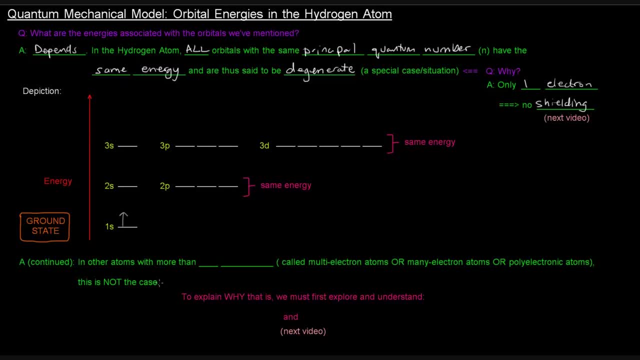 So that's the hydrogen atom. Now, in other atoms with more than one electron, more than one electron, they're called multi-electron atoms, also known as many electron atoms or poly-electronic atoms. They have more than one electron. That's not the case.